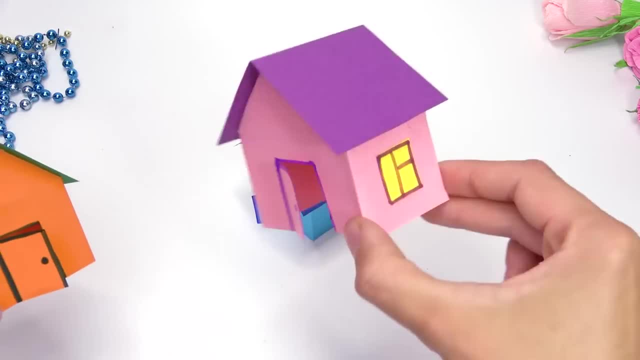 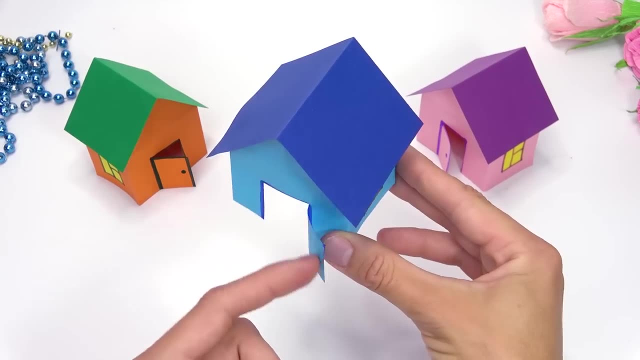 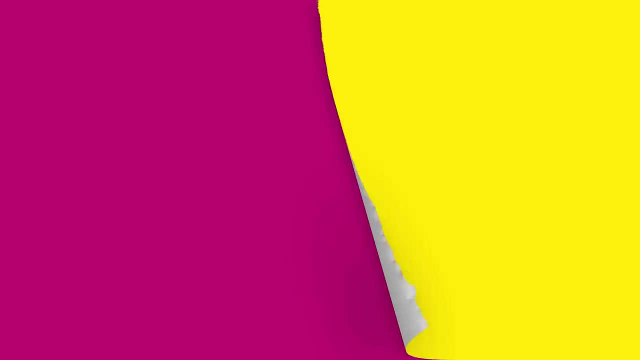 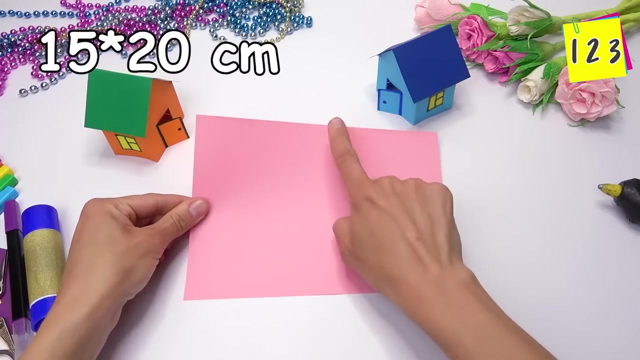 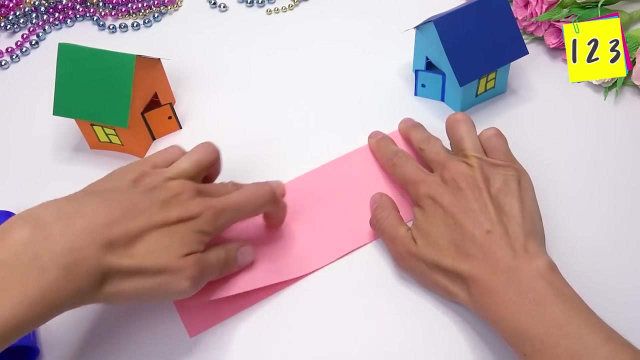 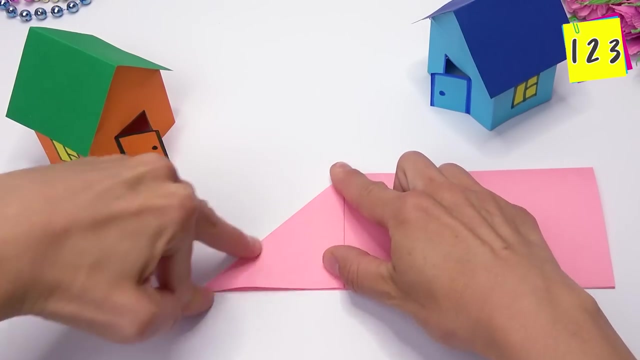 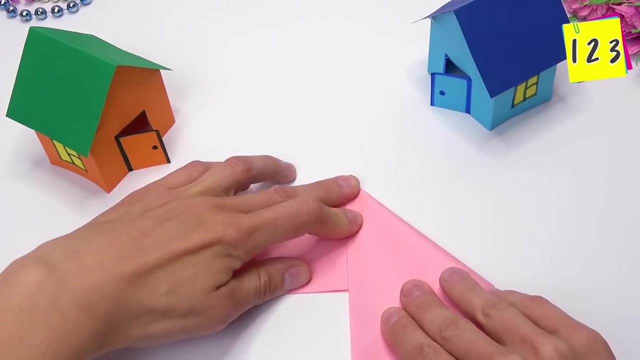 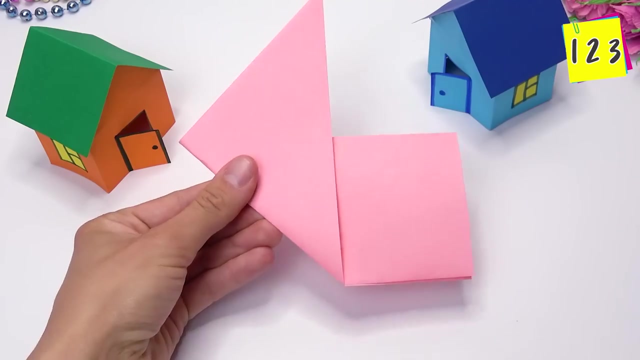 One, two, three Easy paper crafts. The second thing is you have to use the paper. I will show you how to do it now. The third thing is to use the paper and cut it. It is a very important part. 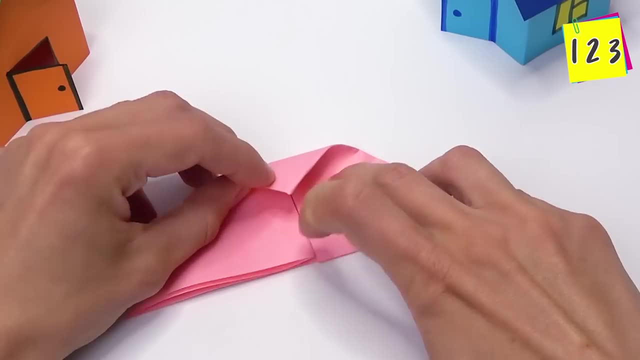 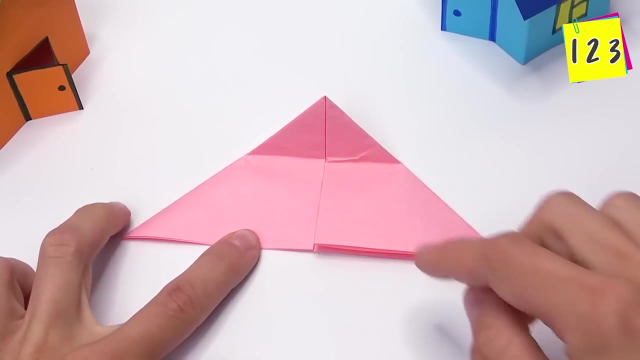 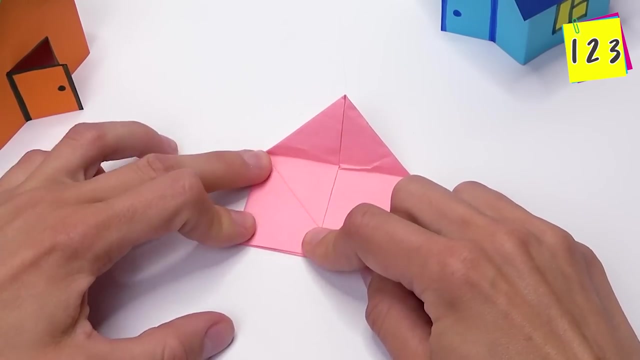 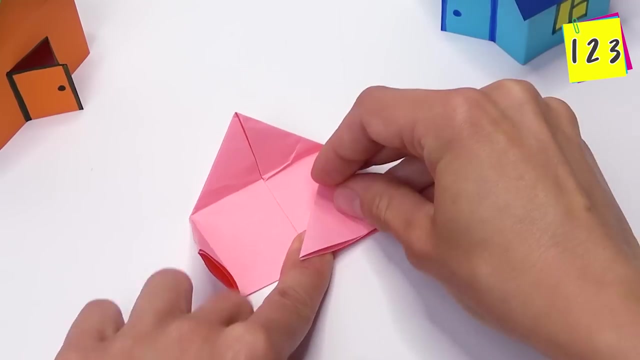 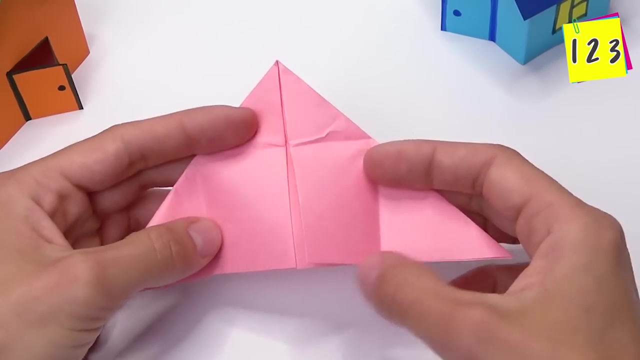 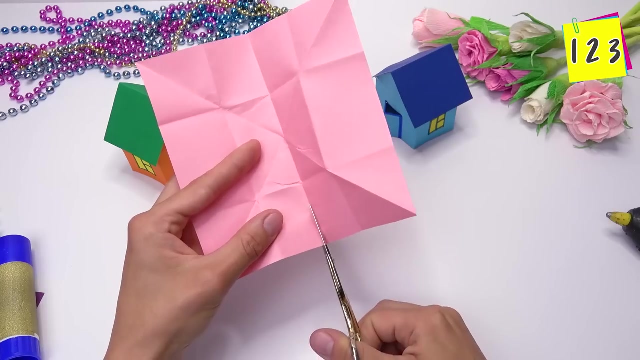 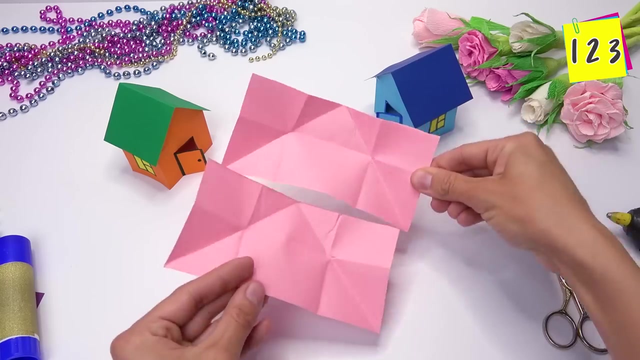 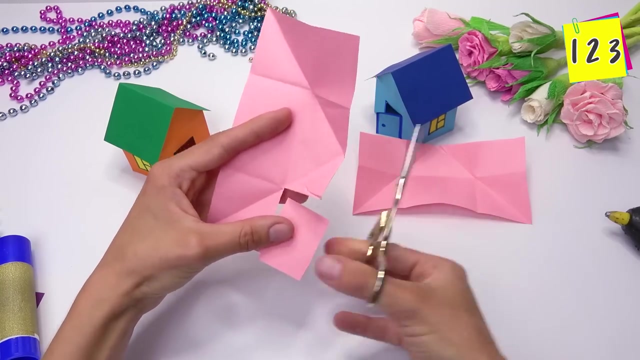 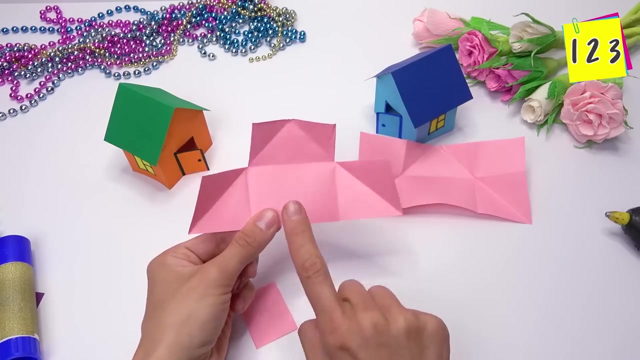 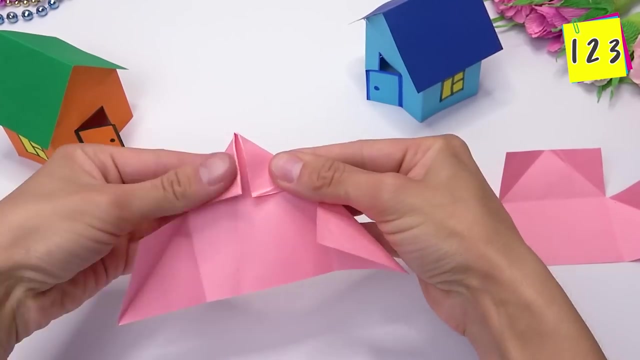 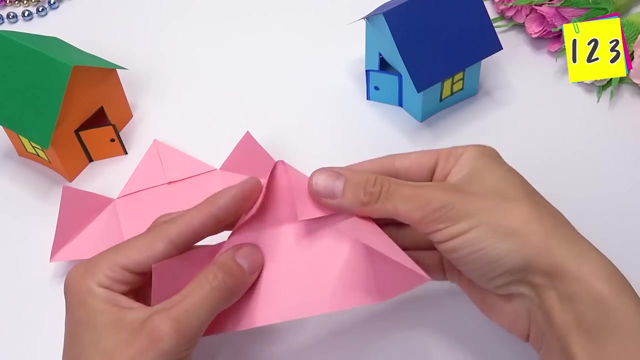 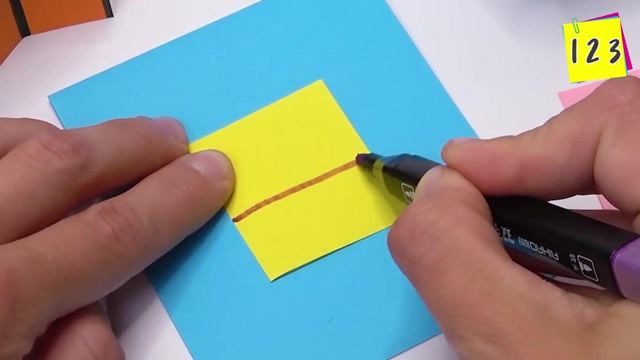 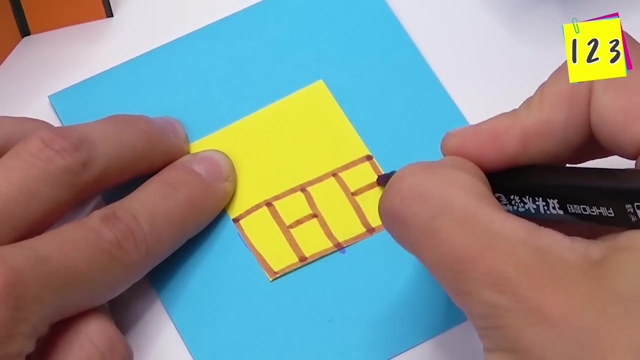 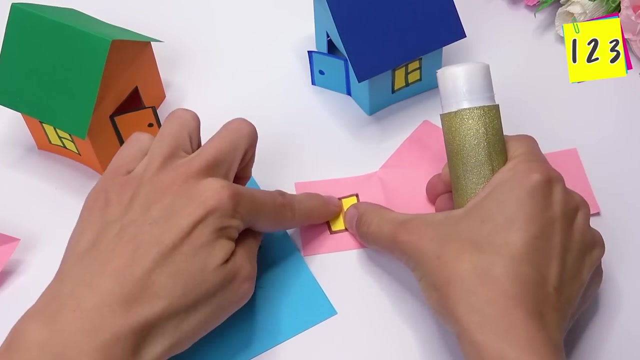 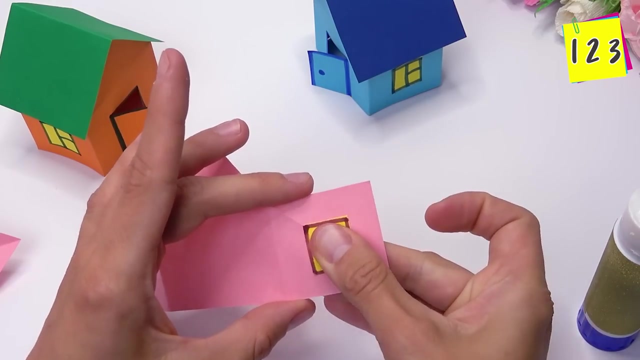 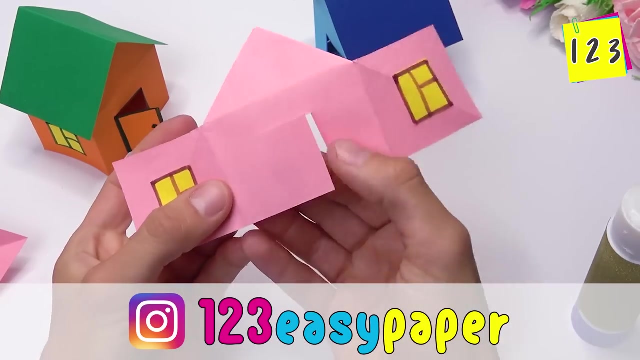 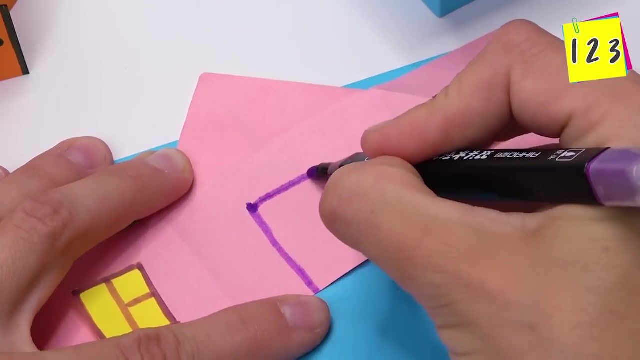 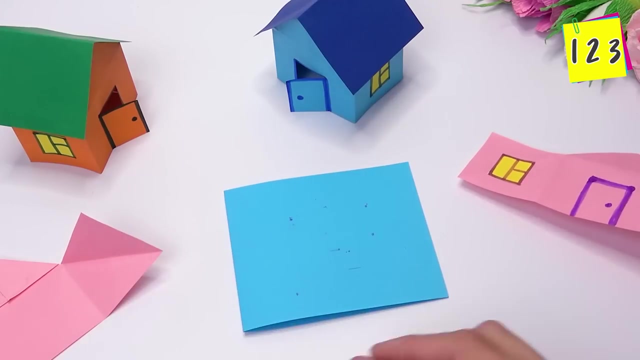 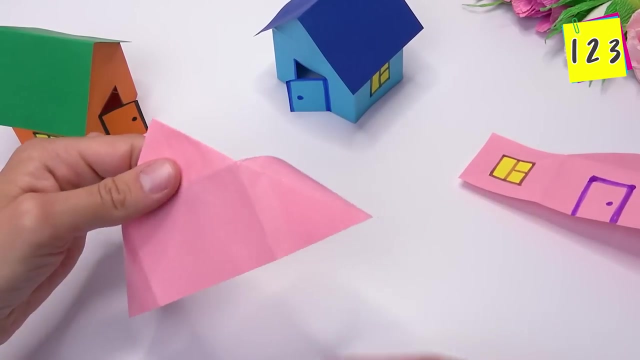 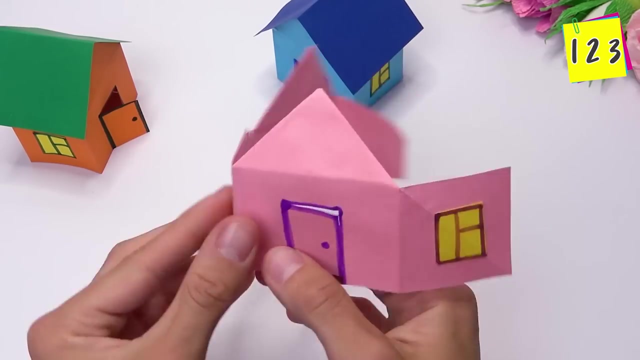 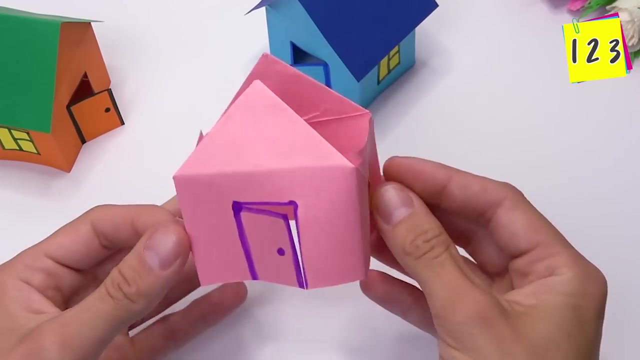 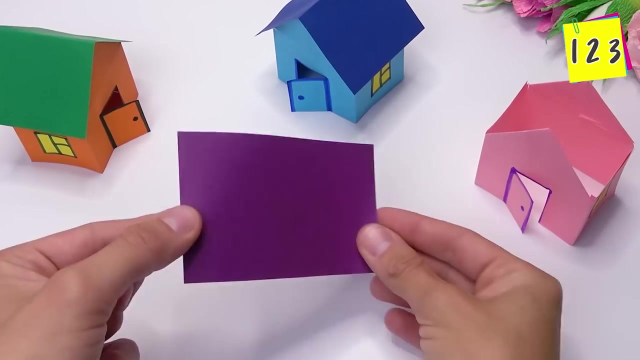 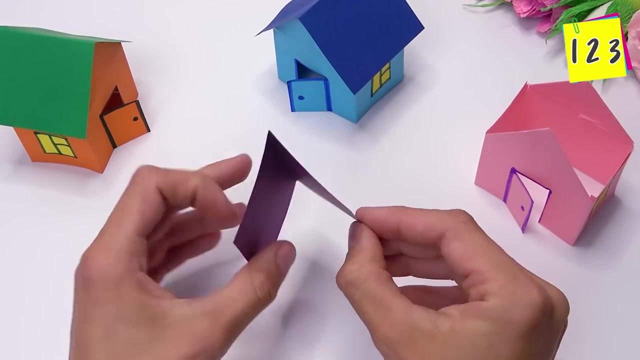 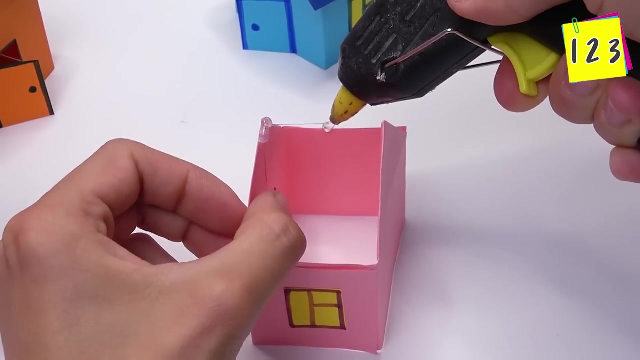 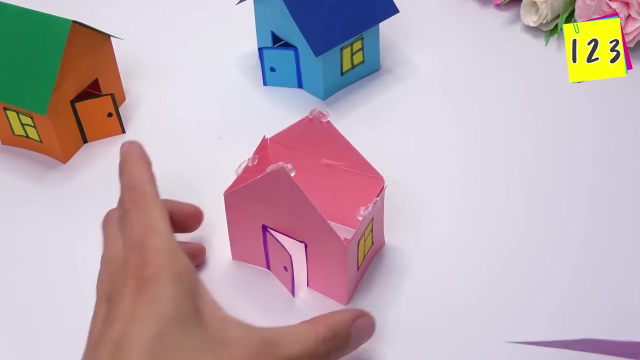 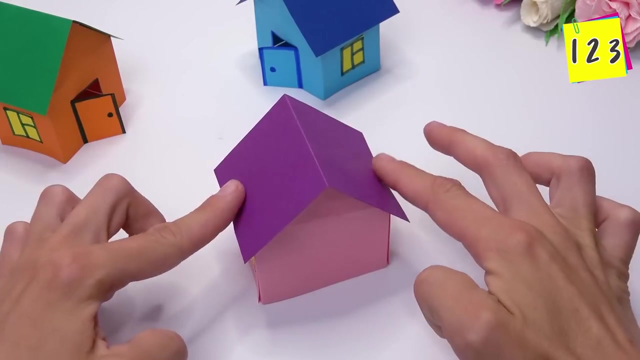 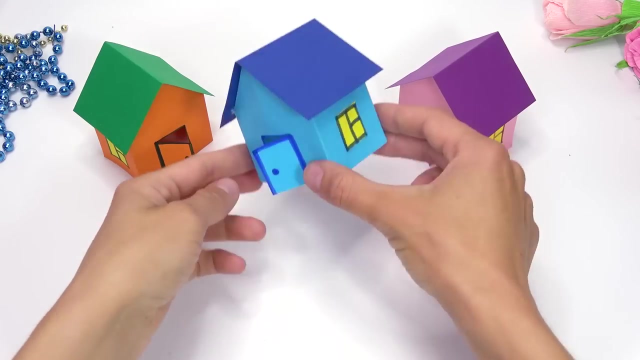 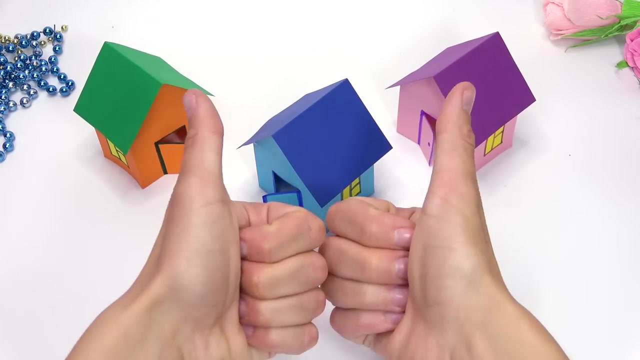